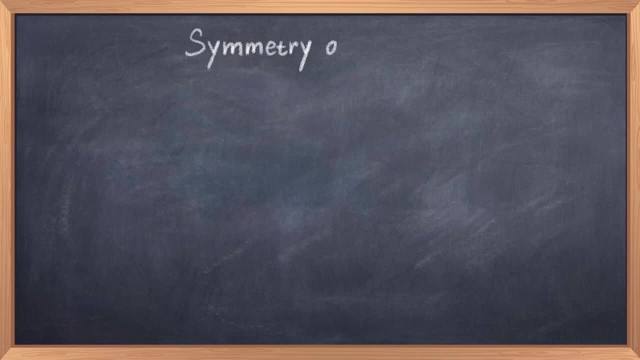 To understand the essence of the issue, we must understand that the standard model is based on gauge theories with certain symmetries that the theory must obey. The symmetry group of a standard model is a rather complicated topic that deserves a video on its own, but the essence is that when you write the Lagrangian of the standard, 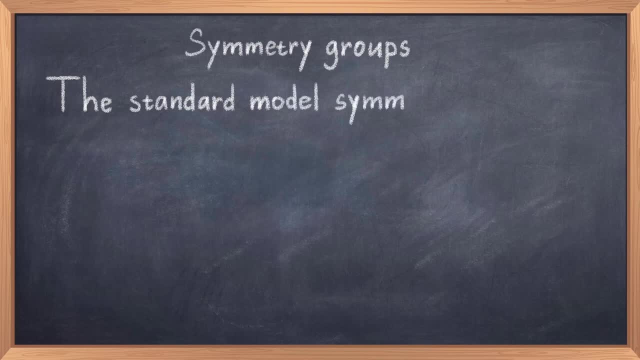 model such that it obeys the underlying symmetries, then we are not allowed to write any mass terms for our gauge bosons. Thus all our force carriers are unaligned. The symmetry of the standard model must be massless. If we wrote mass terms, we would break the symmetry of the standard model, which means 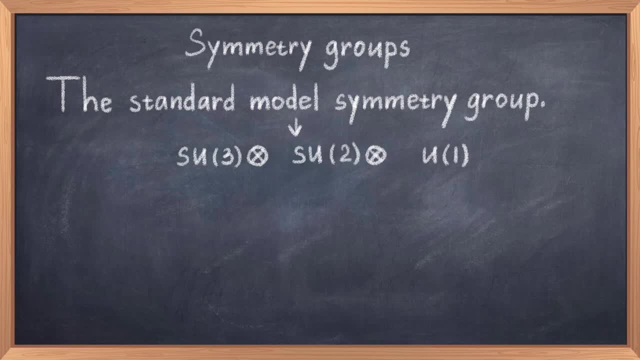 we would break gauge invariance, and this just means that the standard model would be completely useless. The trick is that we can write the standard model Lagrangian such that it abides to the necessary symmetries, but we can write it such that it has a symmetry breaking mechanism. 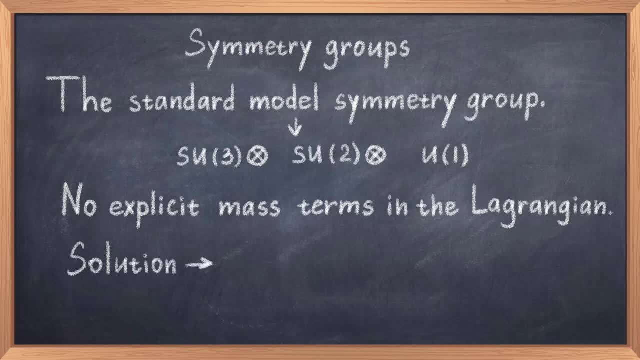 thus the Lagrangian abides to the necessary symmetry, But it has a mechanism. It has a mechanism to then break this symmetry, and this symmetry breaking is what generates the masses of the weak force bosons. This mechanism is called the Higgs mechanism. 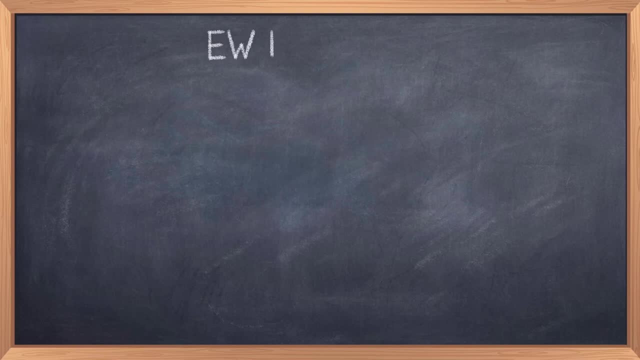 The development of the electroweak theory goes back to the 1960s, when scientists suspected that the weak force and the electromagnetic force were related. On top of that, they were also looking for a way to explain how the force carriers the 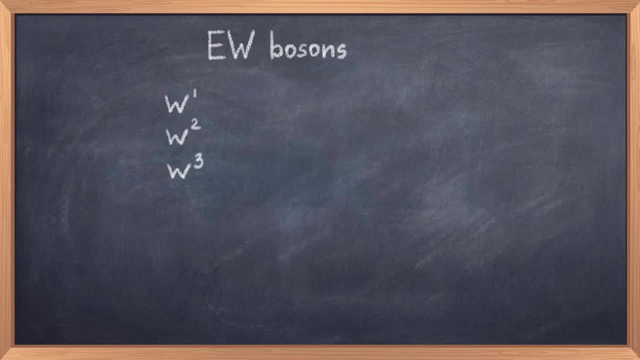 W minus, W plus and the C bosons could be massive without any force. This led to a theory with four massless electroweak bosons called the W1,, W2, W3, and B bosons. Initially, scientists proposed just to manually do a symmetry breaking which would turn three. 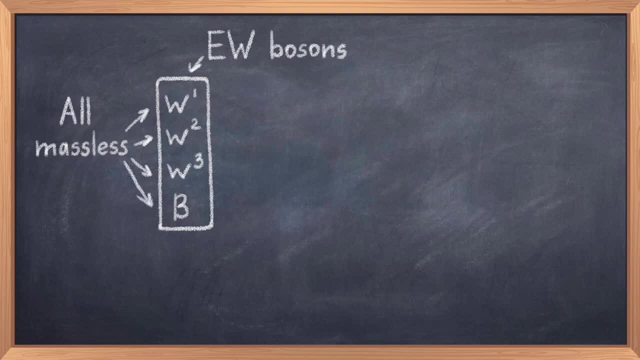 of the bosons massive. but that solution was no good and obviously not natural. The solution came from Peter Higgs, who had earlier proposed a new Higgs field, and this field would have a potential with a potential of 0.5. 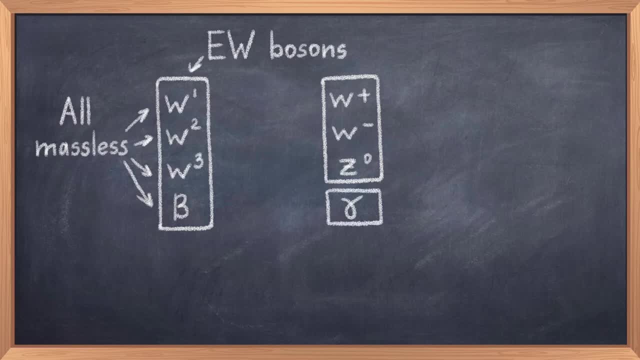 So the solution came from Peter Higgs, who had earlier proposed a new Higgs field, and this field would have a potential with a potential of 0.5.. Then this field produced a particular shape and that potential would spontaneously break. 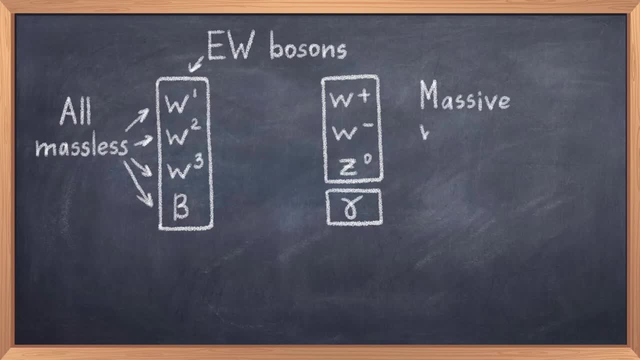 the necessary symmetries to get the correct massive gauge bosons or force carriers. You might think that the W1, W2, and W3 bosons become the weak bosons and then the B boson becomes the photon after the symmetry breaking. but it's more complicated than this. 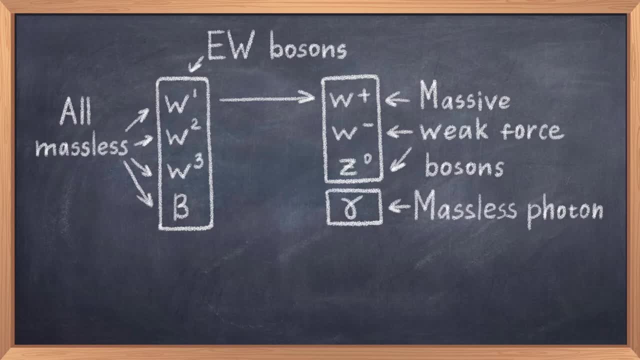 All the ном subsidies in this theory didn't work out. What actually happened is that the W1 and W2 bosons mixed to form the chargeなんです charged W- and W- bosons, and likewise the W3 and B bosons mixed to form the Z boson. 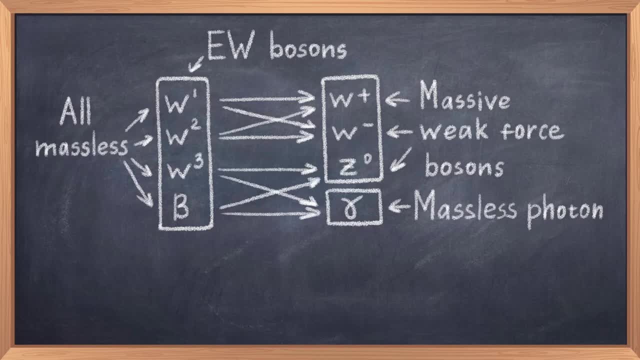 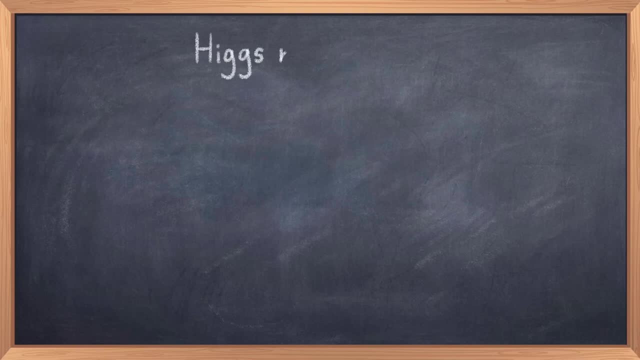 and the photon, But the photon remains massless, while the other particles will become massive. Let us now discuss in more detail how this potential works and how it results in these masses. To do this, we have to introduce something called the vacuum expectation value, or F. 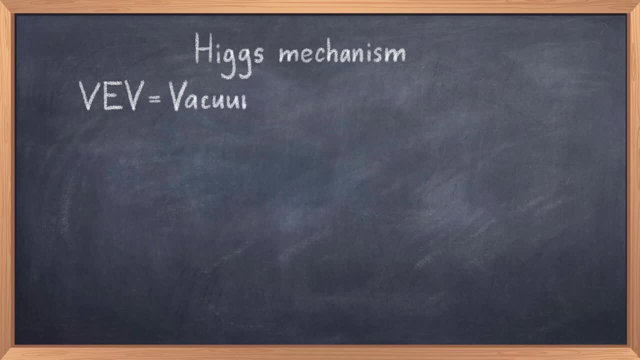 This is the average value of the vacuum of the Higgs field. We often write it just as V, and this is the only mass parameter in the standard model. thus, any fundamental particle with mass is related to the value of the width. Thus, the actual value of the width has a direct impact on the masses of all massive particles. 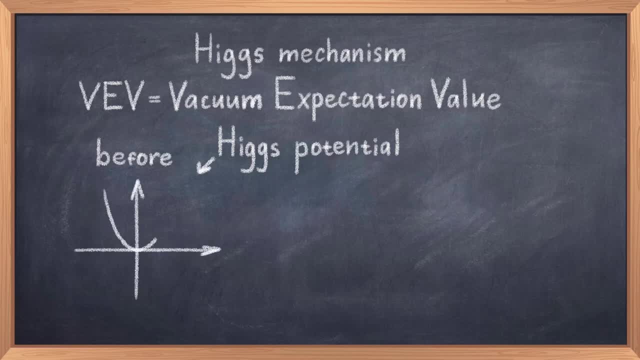 of the standard model. The potential is like a parabola: at energies above 160 GV But at colder temperatures, corresponding to energies lower than 160 GV, this potential changes into the famous Mexican hat potential. Let me just say that 161 GV is incredibly hot and room temperature is many orders of 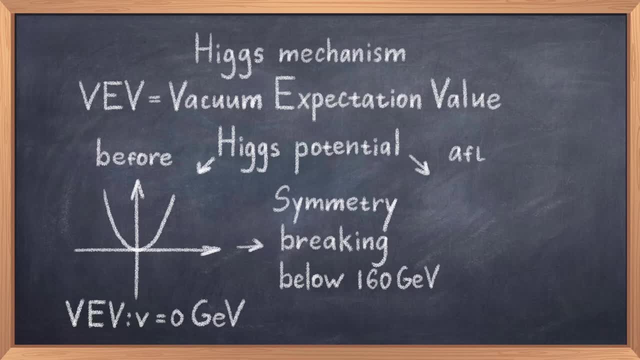 magnitudes less than a GV. Any physical system would like to minimize the energy, so the Higgs field drops into the new minima of the Mexican hat potential. The key here is that the width of the Higgs field is the distance between the mass and 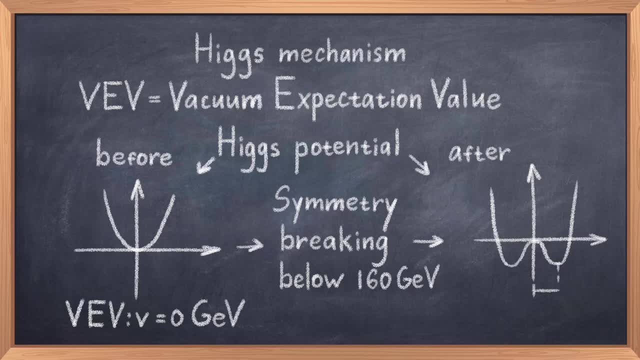 the distance from the center to the Higgs field. In the parabolic potential the Higgs field is at the origin, so the width is zero. But in the Mexican hat potential the Higgs field is now shifted away from the origin. 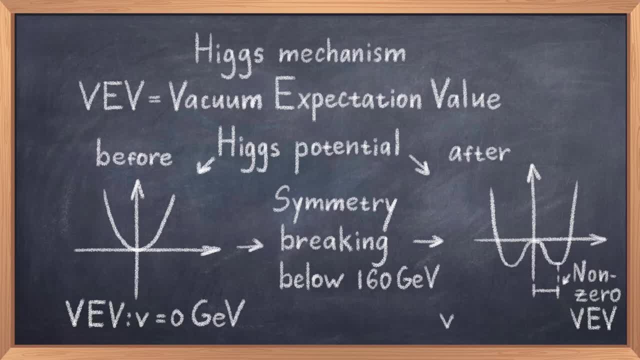 and this displacement on the x-axis leads to the width becoming non-zero. The width actually has a value of 246 GV. This change from the parabolic potential to the Mexican hat potential is the spontaneous symmetry breaking Which leads to the mass of the weak bosons and it gives mass to the Higgs field, which 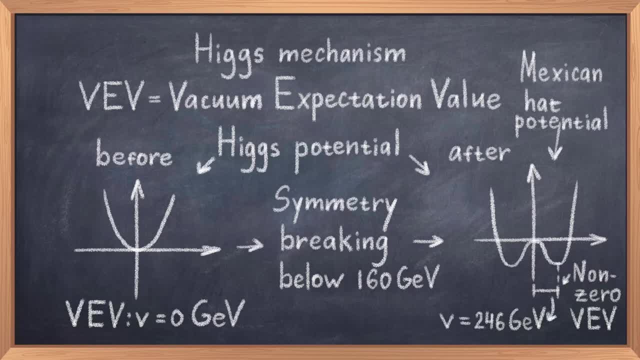 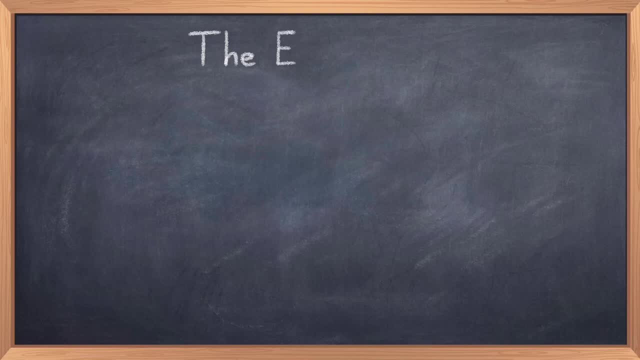 in turn gives mass to all the other fundamental particles. This symmetry breaking is called the Higgs mechanism. Before moving on to show you exactly how the masses appear, let us talk a bit more about symmetry breaking from the point of view of the symmetry groups. 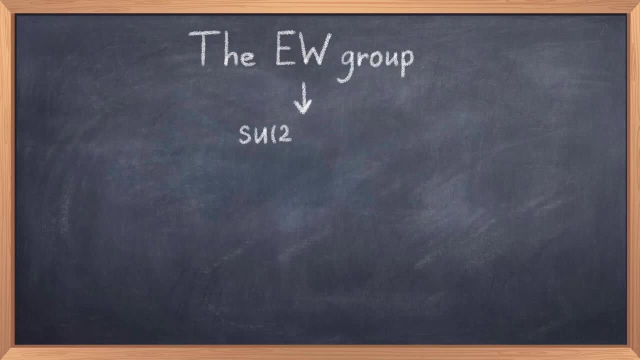 The group involved in the electromagnetic force is called U1, and this group has one so-called generator. What is important here is that generator equals bosons. thus, one generator means one boson. This is why the electromagnetic force has just one boson, namely the photon. 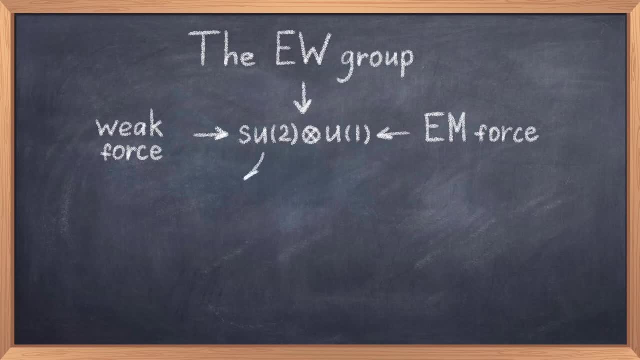 The group involved in the weak force is called SU2, and it has three generators. This therefore means that we have three bosons associated with this force. To create the electroweak theory, we obviously must combine these two groups. The first group is the weak force. 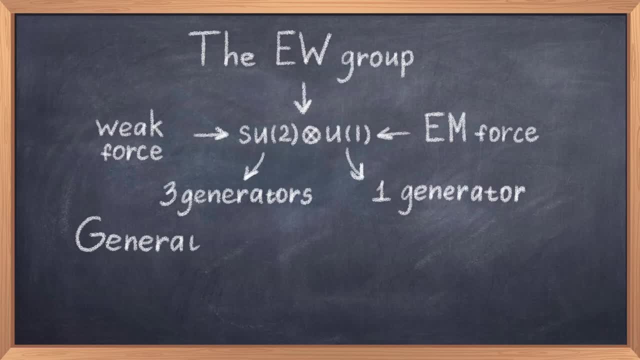 The second group is the weak force. We combine these two groups to form a combined theory. thus, the group of the electroweak theory is the product of the group of the weak and the electromagnetic force. This gives us the group SU2, cross U1.. 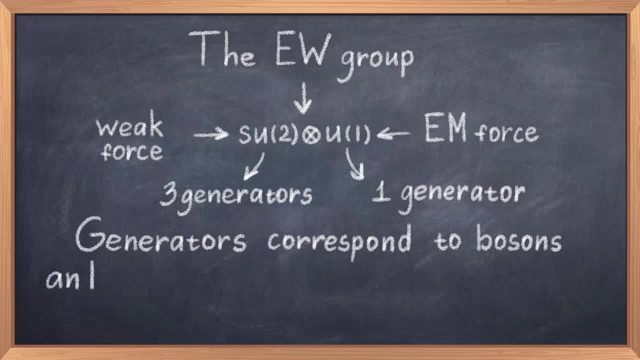 When we talk about symmetry breaking in the case of the Higgs mechanism, we are talking about the breaking of the generators of the SU2 symmetry group, because it has three generators and they all get broken by the Higgs mechanism. Then we get three massive weak bosons. thus, a broken generator means a massive boson. 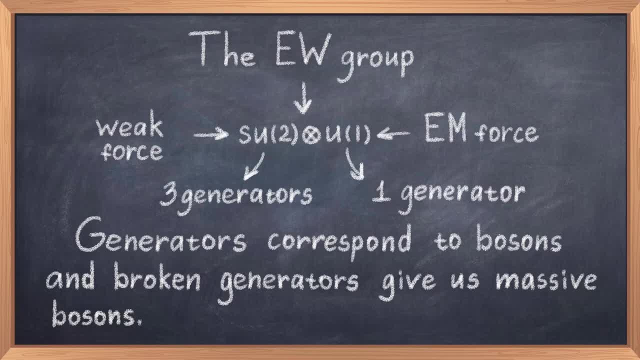 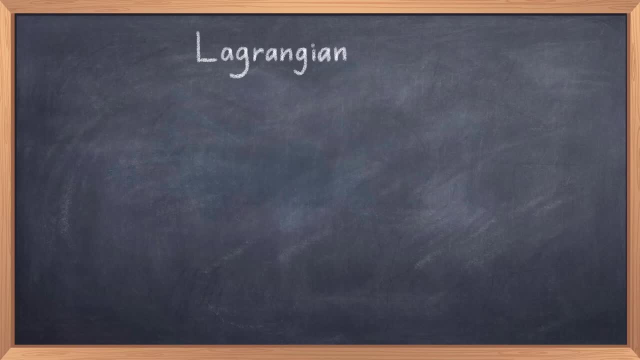 and since the U1 group remains unbroken, then the photon stays massless. Now let us look at the math of the situation. The Lagrangian for the electroweak theory has many terms, but one term is instructive, to show how the symmetry breaking works. 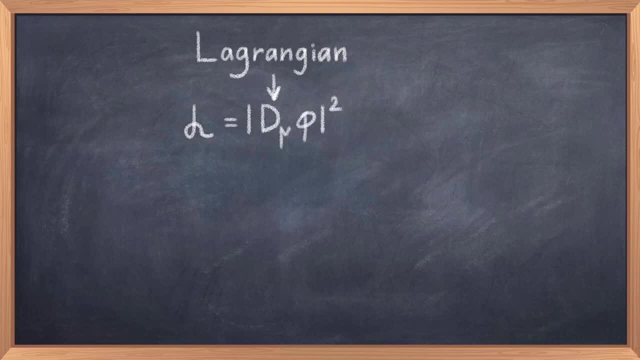 This term is written Before symmetry breaking as: L is equal to d mu, phi and all that squared where phi is the Higgs field and the d mu term is the covariant derivative of the SU2 cross U1 symmetry group. This term can be written as: d mu is equal to a half and, in parenthesis, two partial. 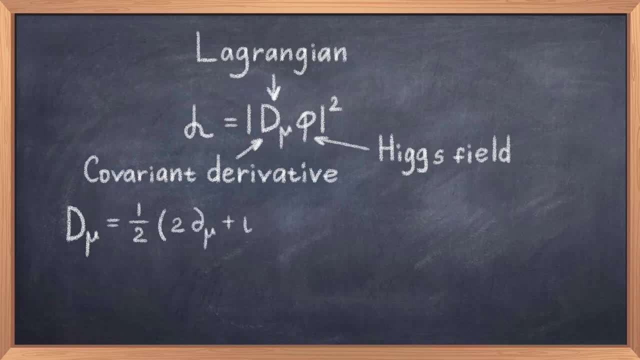 mu plus i g prime. b mu plus i g sine. This term can be written as: d mu is equal to a half and, in parenthesis, two partial mu plus i g prime b mu plus i g sine. The other term for symmetry breaking is the sigma i W i mu. 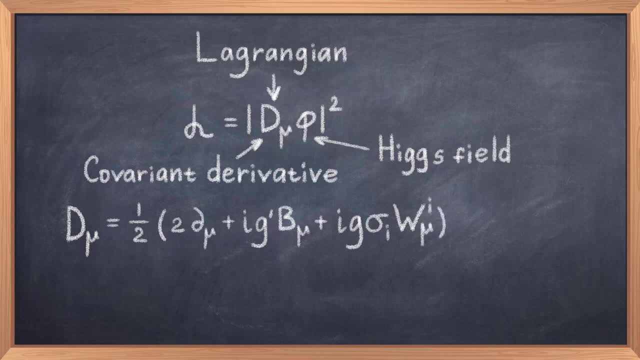 Here we just focus on the last two terms. We first note that the U1 gauge field is called B mu, which gives us the B boson of the unbroken electroweak theory. The coupling constant of this field is G prime. 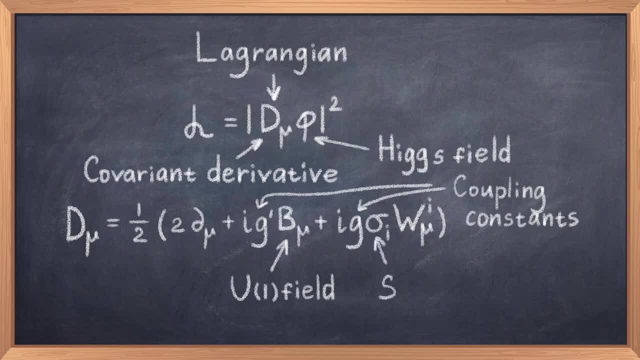 In the next term. we have 3w bosons as the index. I goes from 1 to 3.. The coupling for the bosons is g. The sigma i term is the three generators of the SU group which are all broken by the symmetry breaking. 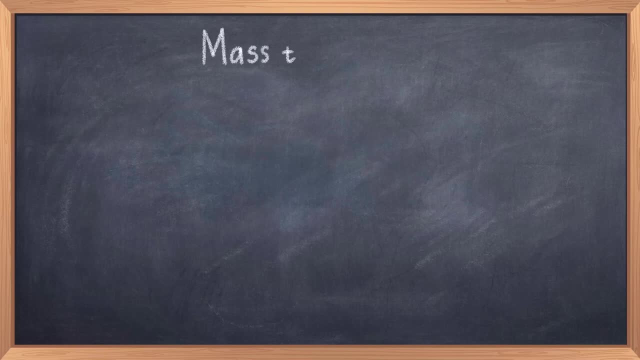 Now the last thing we will discuss is how symmetry breaking gives us mass terms. What we will do is to insert the value of the Higgs field after symmetry breaking into the Lagrangian presented in the previous slide. First, we write the Higgs field in a symmetry broken state, as phi is equal to 1 over the square root of 2,. 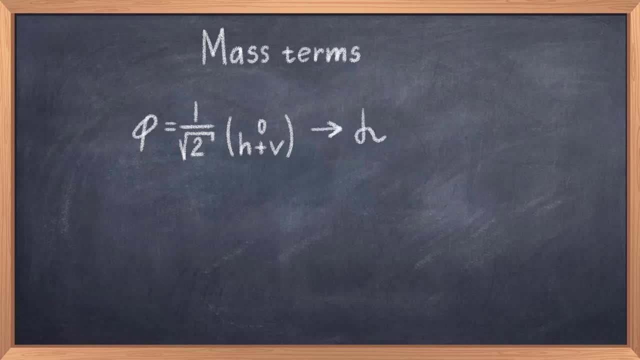 and then the upper value of the vector is 0, and the lower value is h in the Higgs field plus v. Then we plug this into the Lagrangian: it is equal to d mu phi, and that squared. And then we do a lot of math and get a lot of terms, but we are interested in the masses. 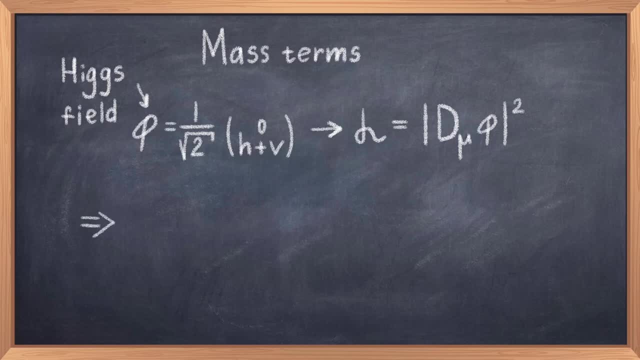 As discussed before, the w minus and the w plus boson come from the w1 and w2 bosons. These bosons have the same mass but just opposite charts, and we thus get the two terms a half mw squared, parenthesis w mu1 squared plus w mu2 squared. 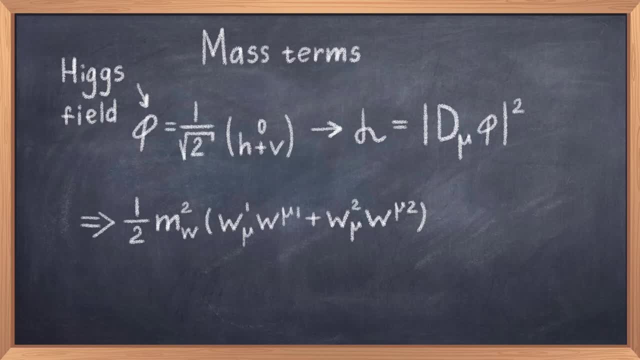 where the mass of the weak force w bosons is mw equal to a half gv, And we can explicitly see here that the mass depends on the vacuum expectation value of v and the coupling. Something similar happens for the c boson, but because of the mixing. 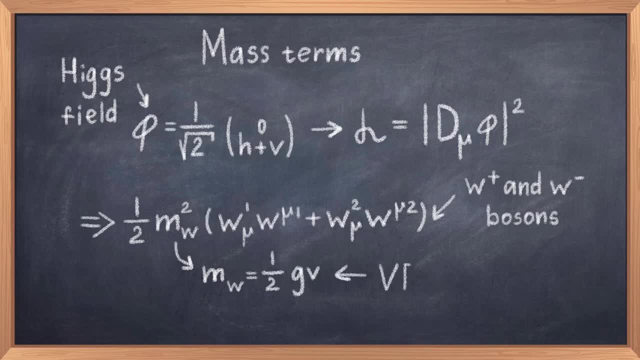 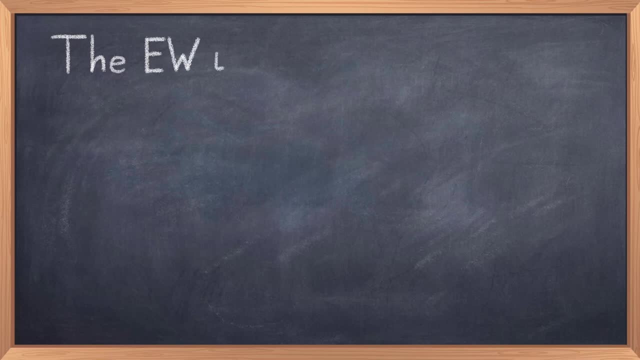 there is a bit more work to do to figure out the mass term, But this illustrates how we get the mass term from the Lagrangian. This video has focused on the electroweak theory and how it explains the mass generation of the weak bosons.